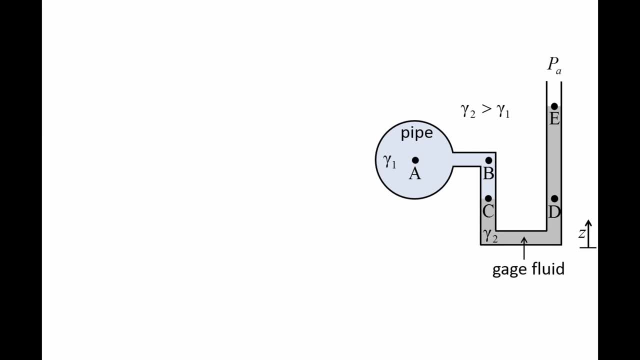 Point E is at the interface between the gauge fluid and the atmosphere. The vertical distance between points A and C is h1 and the vertical distance between points D and E is h2.. The pressure at point A is equal to the pressure at point B because those two points are at the same elevation in a continuous fluid. 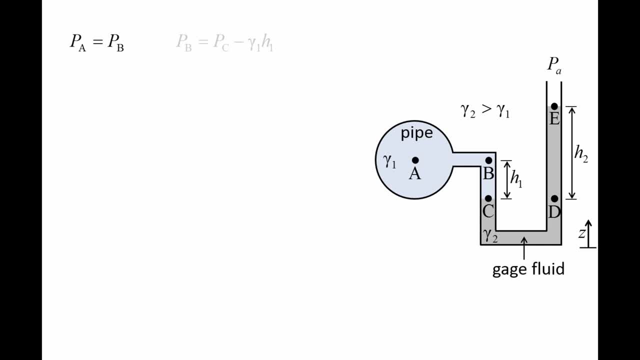 Now we need the pressure at point B. The pressure at point B is less than the pressure at point C by the amount gamma1 times h1.. So now we need the pressure at point C. The pressure at point C is equal to the pressure at point D. 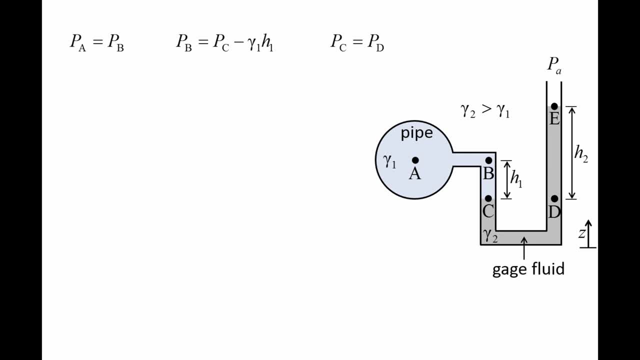 because those two points are at the same elevation in a continuous fluid, Both points are in contact with the gauge fluid. The pressure at point D is equal to the pressure at point E, which is the ambient pressure plus gamma2 times h2.. 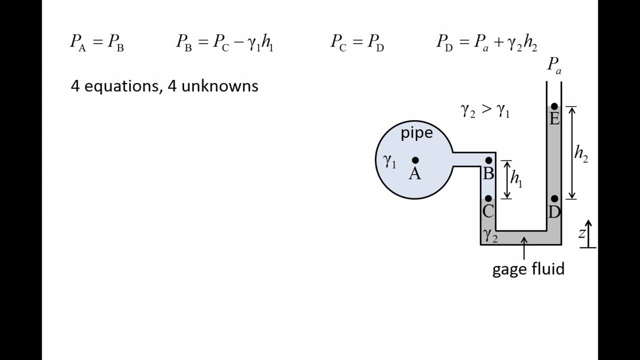 We have four equations and four unknown pressures: The pressure at points A, B, C and D. We can solve these equations to find the absolute pressure at point A, which is the ambient pressure plus gamma2 times h2, minus gamma1 times h1.. 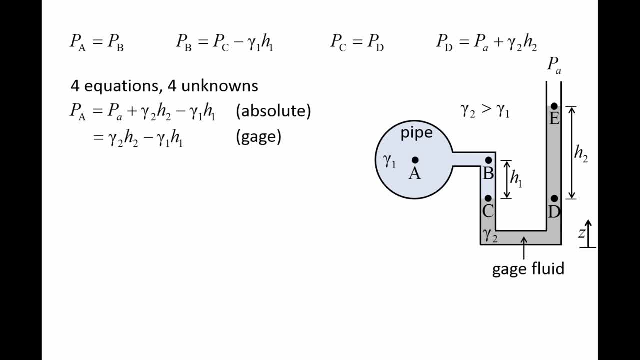 For the gauge pressure, we would subtract the ambient pressure. Instead of solving a set of equations, we can use a shortcut to find the pressure at point A. We start at the far end of the manometer and work our way toward point A. 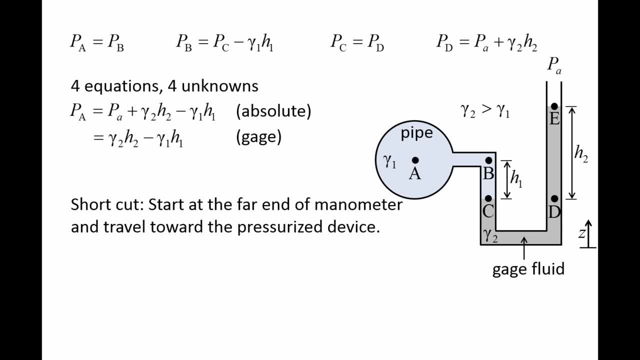 As we travel along the manometer, we follow three rules. We will add a factor of gamma times h when moving downward through a continuous fluid, We will subtract a factor of gamma h when moving upward through a continuous fluid And we can jump horizontally between adjacent sections of the tube. 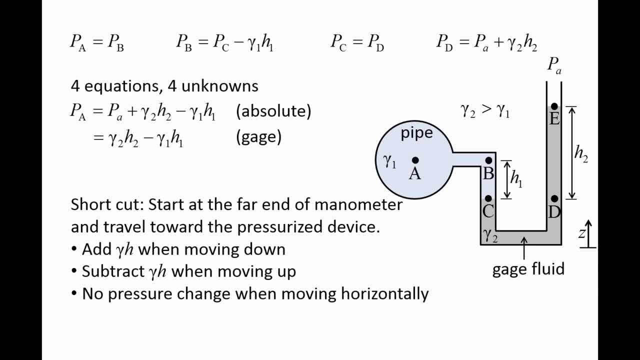 if the fluid is continuous between the two points. So let's start at point E, where the pressure is the ambient pressure. As we travel downward from point E to point D, we add gamma2 times h2. Then we jump across horizontally from point D to point C. 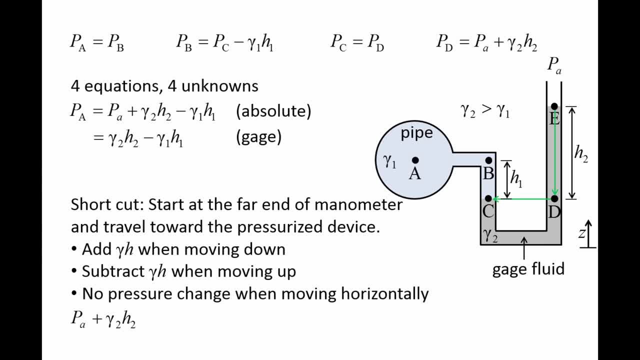 which is allowed, since both points are in contact with the gauge fluid And as we jump from point D to point C, the pressure does not change because they are at the same elevation. Next, we travel upward from point C to point B and subtract gamma1 times h1. 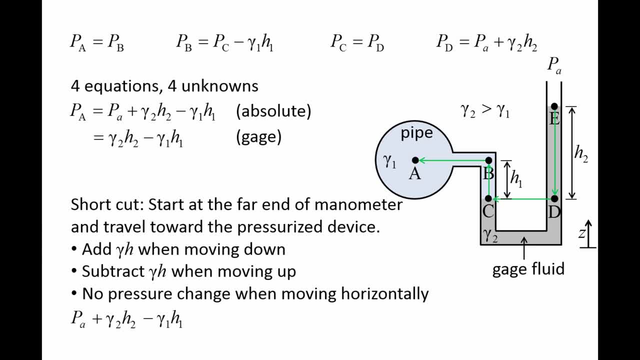 And, finally, there is no pressure change as we move horizontally from point B to point A. Now that we have reached our destination, we can set the entire left side equal to the pressure at point A And notice that we obtain the same equation as when we solved the set of four equations above. 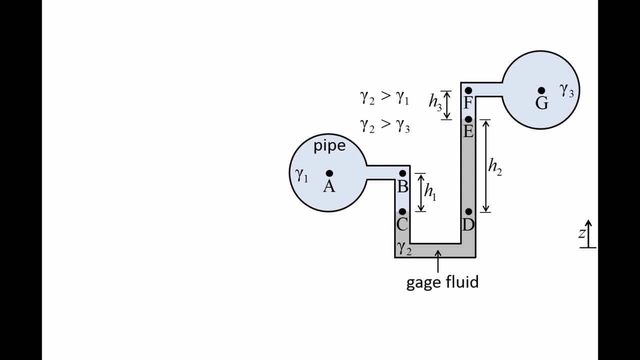 The U2 manometer also can be attached to another device instead of being exposed to the ambient environment, And here we connect the end of the tube to another device, perhaps a different pipe or a different section of the same pipe. Point E now corresponds to the interface between the gauge fluid and the fluid in the pipe. 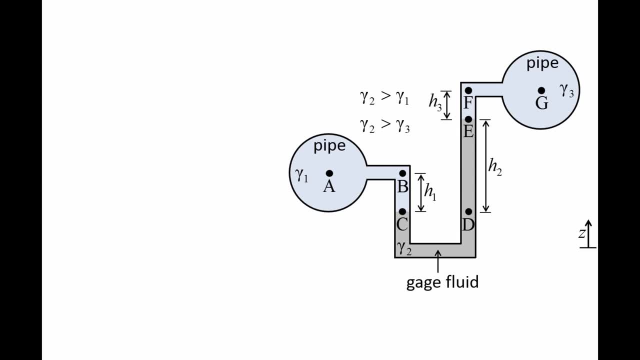 which has a specific weight of gamma3.. For this particular setup, the specific weight of the gauge fluid- gamma2, needs to be greater than gamma1 and gamma3.. Point G corresponds to the point in the center of the pipe and point F is at the same elevation as point G. 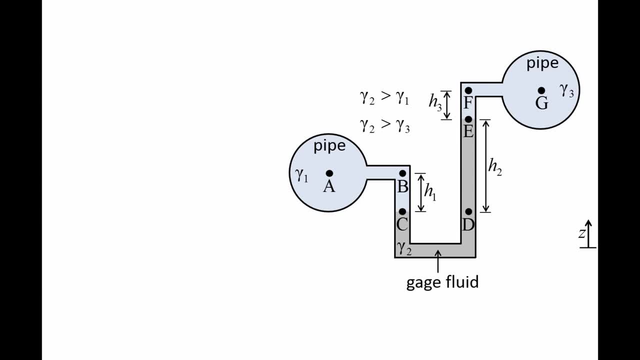 The vertical distance between points E and F is h3.. Let's use the shortcut method to find the pressure difference between the pipe on the left and the pipe on the right. We start at point G, where the pressure is PG. We move horizontally to point F and there is no change in pressure. 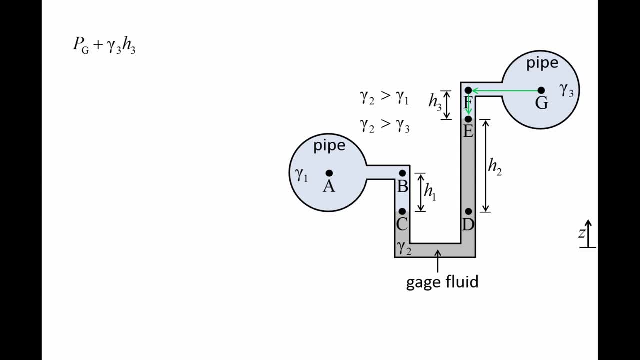 As we descend to point E, the pressure increases by gamma3 h3.. As we further descend to point D, the pressure increases by gamma2 h2.. Now we jump across to point C with no change in pressure. This jump is allowed because both points C and D are in contact with the gauge fluid. 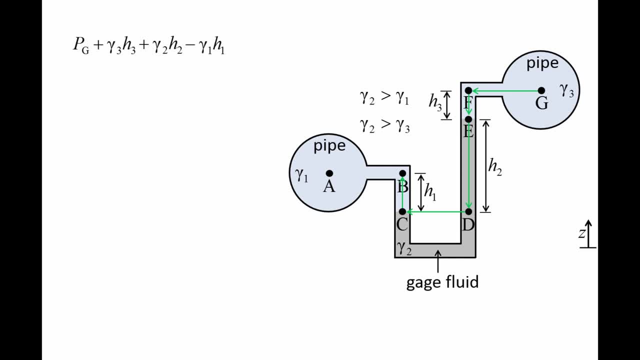 As we move upwards to point B, the pressure decreases by gamma1, h1.. And finally, we move horizontally from point B to point A with no change in pressure. We've arrived at our destination and set the left side of the equation equal to the pressure at point A. 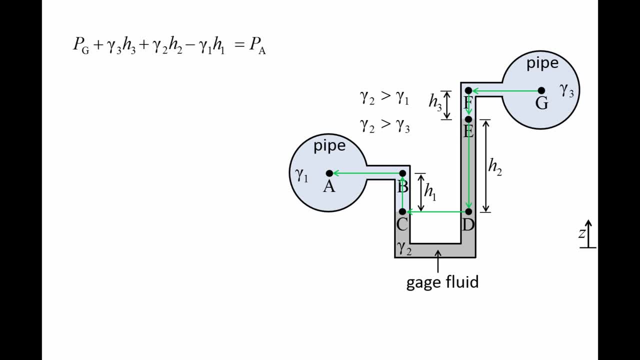 Usually it will be easy to look up the specific weights gamma1,, gamma2, and gamma3 in a fluids textbook or elsewhere, and it would be easy to measure the heights h1,, h2, and h3.. If that is indeed the case, we have one equation, but two unknowns: the pressure at point A and the pressure at point G.